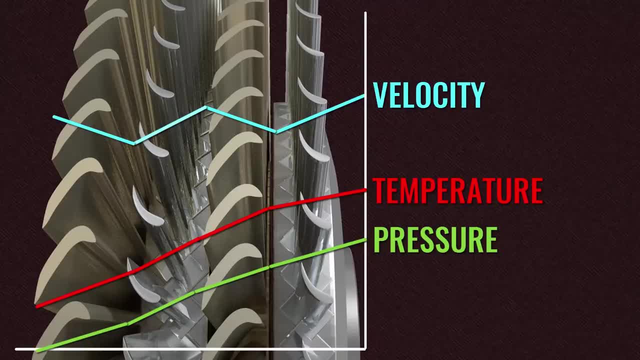 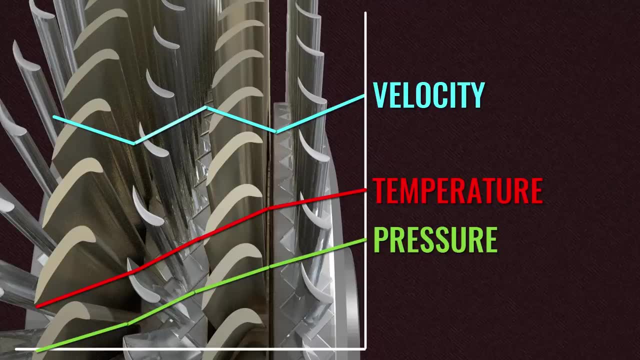 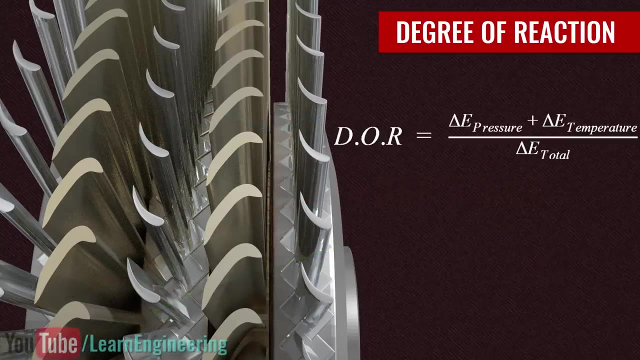 After that, another nozzle set is added. Many such sets are used in a steam turbine. There is an important term while designing steam turbines, namely degree of reaction. This term is calculated by dividing pressure and temperature energy by the total energy change in the rotor. 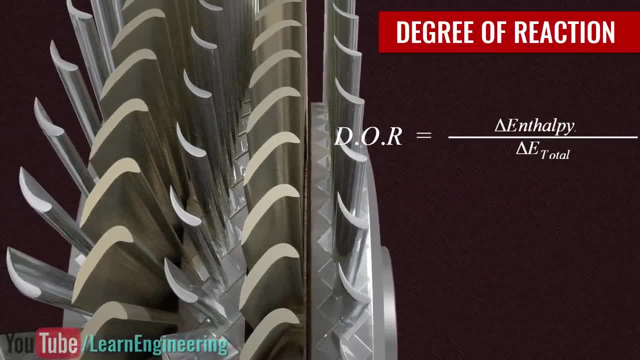 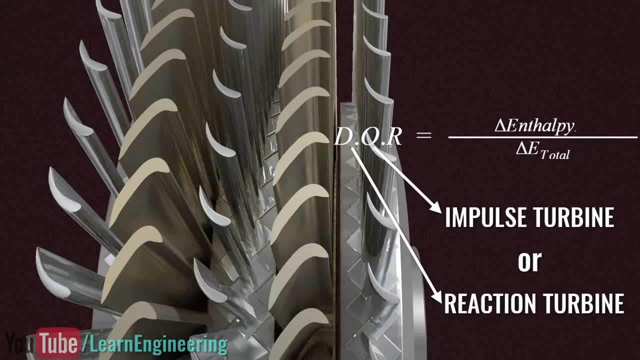 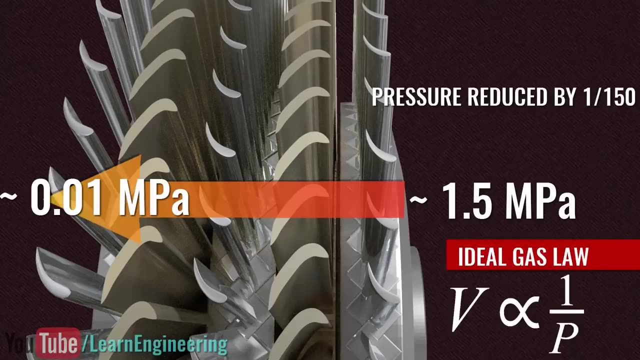 Pressure and temperature energy together is called enthalpy. The degree of reaction decides what type of steam turbine it is. As the pressure of the steam undergoes a drastic reduction during steam turbine operation, its volume increases proportionally. To accommodate such an expanded steam we have to increase the flow area. 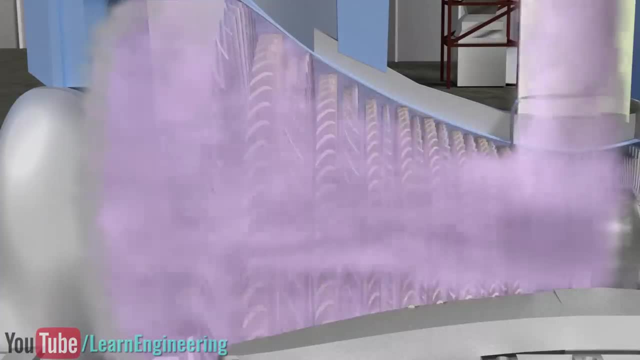 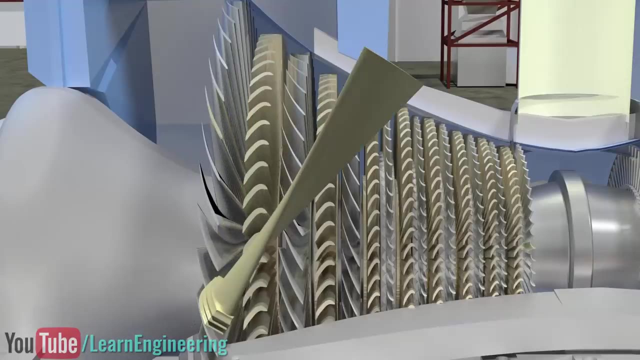 Otherwise the flow speed will become too high. This is the reason why the steam turbine blades are too long towards the outlet. You can see how long the last stage turbine blades are compared to the first stage blades. The tips of such long blades will have very high velocity compared to the root. 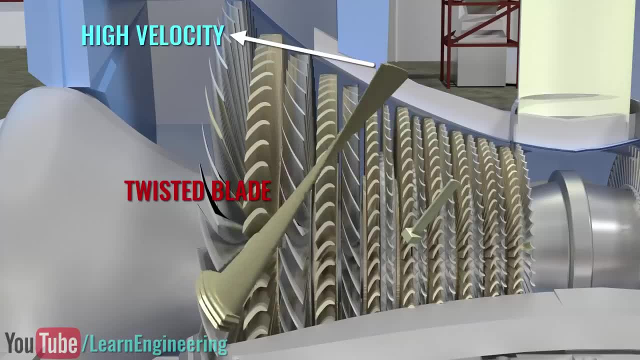 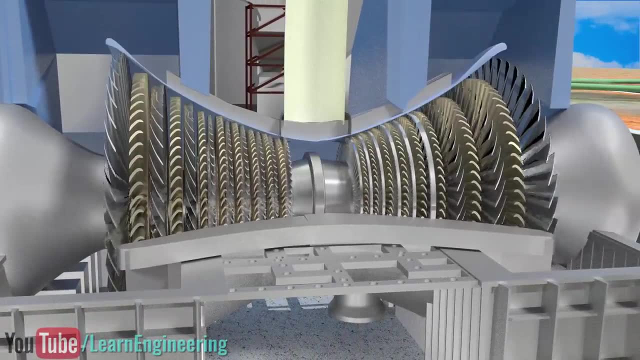 A twist is given to it so that all blade cross sections will remain at an optimum angle of attack. This kind of large turbine uses two such symmetrical units. You can see how the steam is equally divided between the top and the bottom of each of these units. 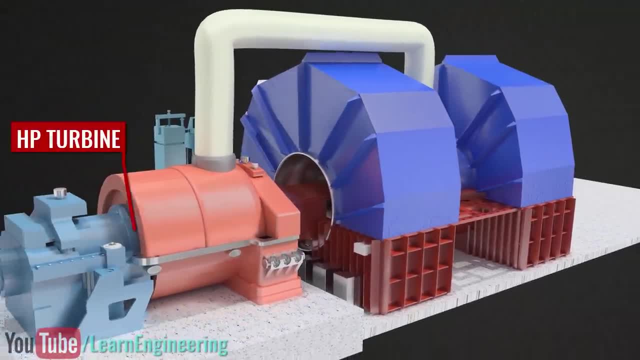 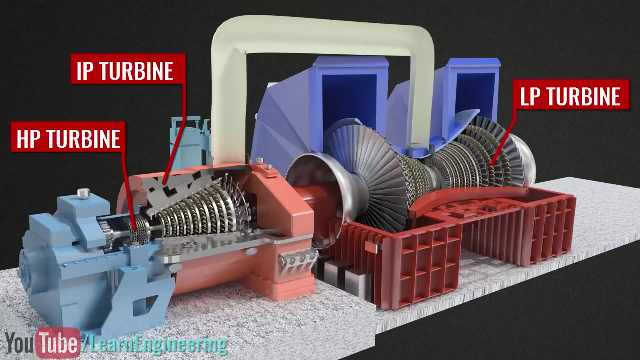 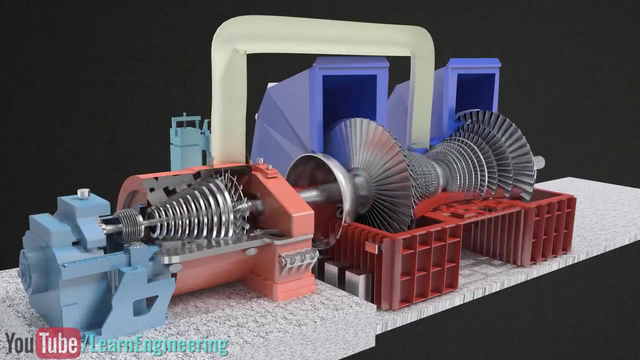 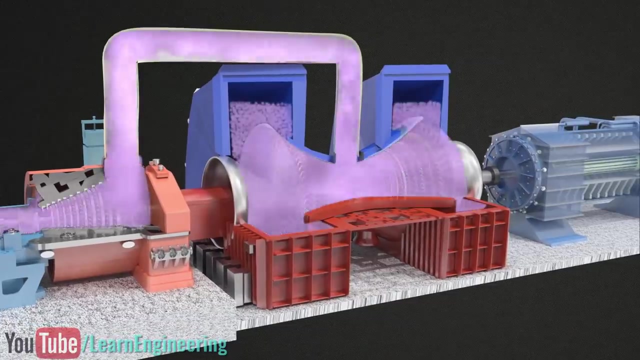 High capacity power plants use different stages of steam turbines, such as high pressure turbine, intermediate pressure turbine and low pressure turbines. All these units are attached to a single rotating shaft. The shaft, in turn, is connected to a generator. This is the reason why the steam turbine blades have such different stages is quite interesting. 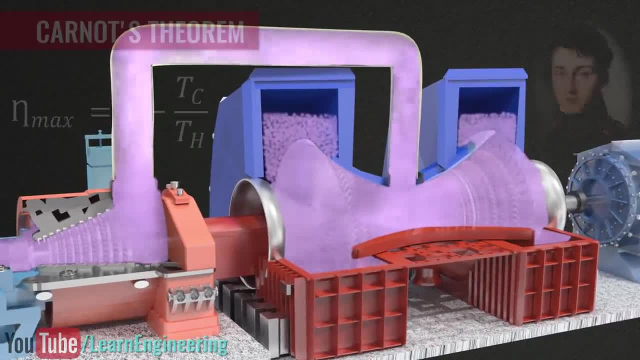 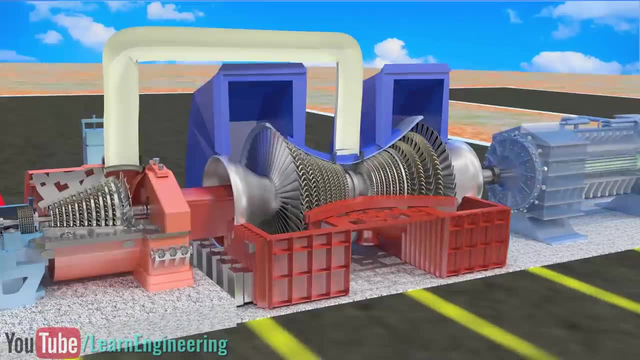 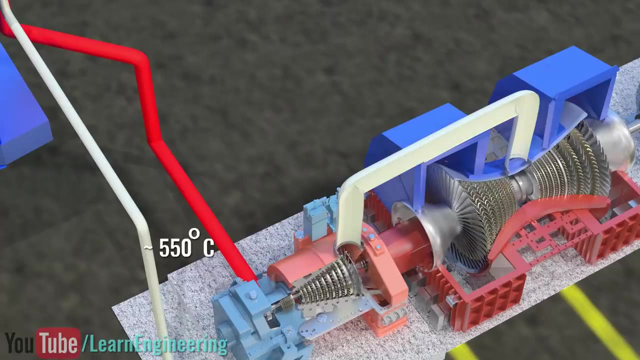 With greater steam temperature comes greater power plant efficiency. This is according to the second law of thermodynamics, But we cannot have temperature greater than 600 degrees Celsius, since the turbine blade material will not withstand temperature more than that. Temperature of the steam decreases as it flows along the rows of the blade. 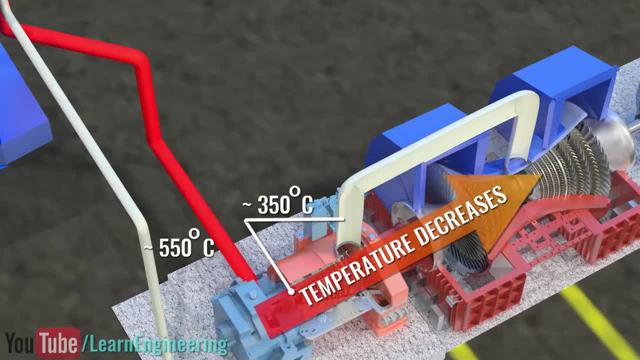 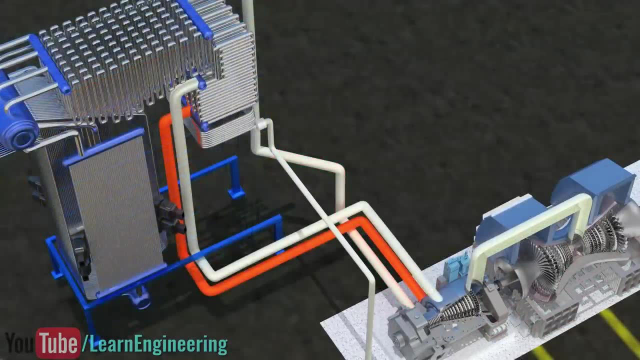 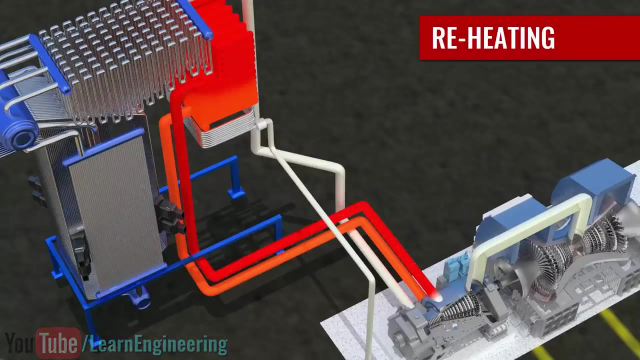 Consequently, a great way to increase power plant efficiency is to add more heat after the first stage. So after the first stage, the steam is bypassed to the boiler and more heat is added. This is known as reheating. This will increase the steam temperature again, leading to higher power plant efficiency and output.